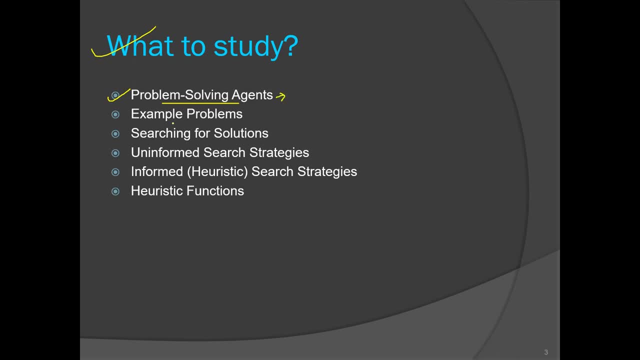 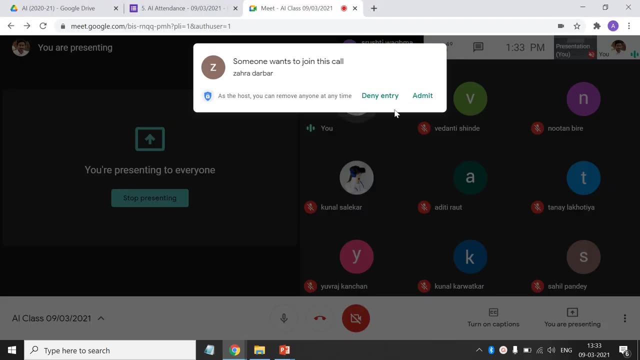 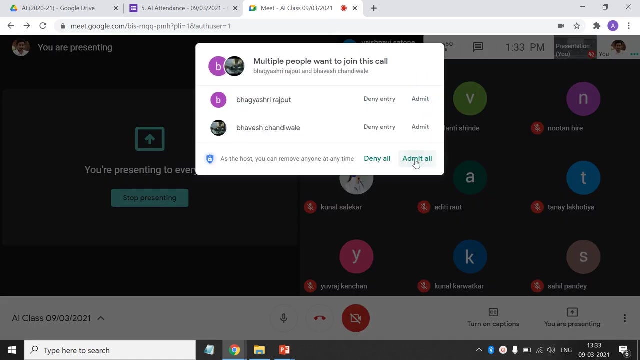 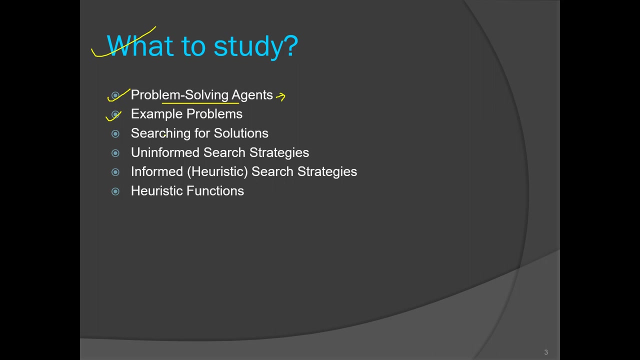 the sequence of action to achieve their goals. then we'll see different example problems. here we are going to discuss different puzzles. so here we'll try to solve different puzzles and then searching for solutions. so we are going to study different search algorithms. so here we are going to see means, how to measure the performance of 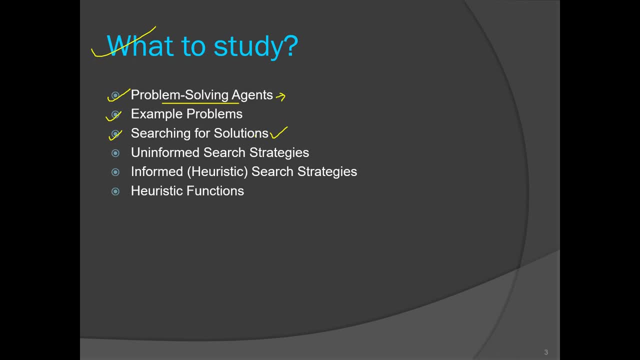 those search algorithms in terms of time, complexity, space complexity, optimality, completeness, those parameters will study here. then we are going to study these two search strategies, that is, uninformed and informed- okay. so in uninformed search strategy, will will not have any information available, okay. and in inform such strategies, we will have some heuristic, we will have. 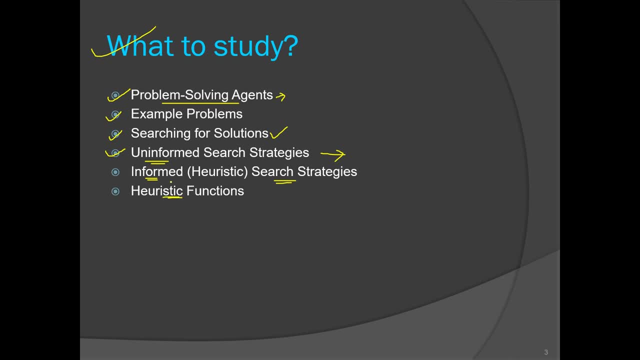 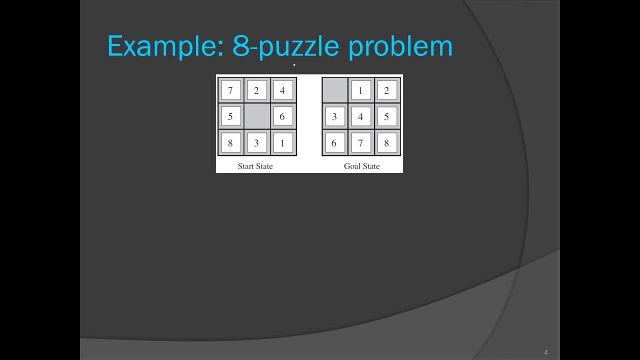 some information in terms of heuristic function. okay, that will guide during the guide us during the search, searching. okay, so this is the content of this second unit. okay, before moving ahead, we'll see eight puzzle problem. so I think you might be knowing this eight puzzle problem. in eight puzzle problem we have 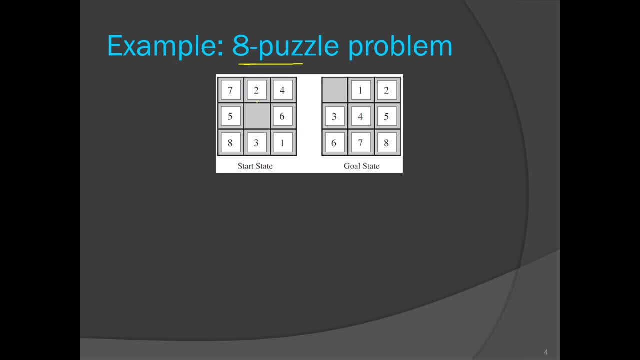 this 3 by 3 grid, okay, and 8 tiles are placed and these tiles are numbered from 1 to 8. these tiles are numbered from 1 to 8. okay, so we will start with any state okay and in each move i will be moving a tile. 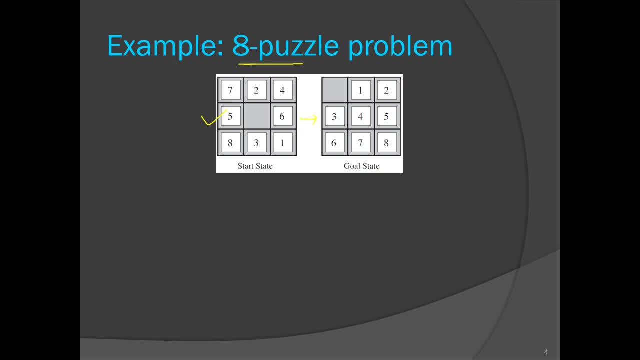 okay, and so as to reach to this goal state. okay, now for different problem goal state can be, so i can give a different goal state to my opponent for the next game. okay, i can give him a goal state like he has to reach to this goal. okay, so every example will have different, different. 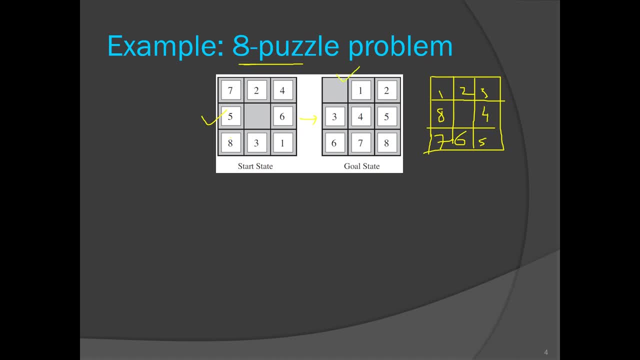 goal state. so this is the goal state for this example and this is the start state. Start state can be again anything. So I am denoting a start state with the help of S0 and goal state with the help of SG. So now my initial state is S0.. Now which? 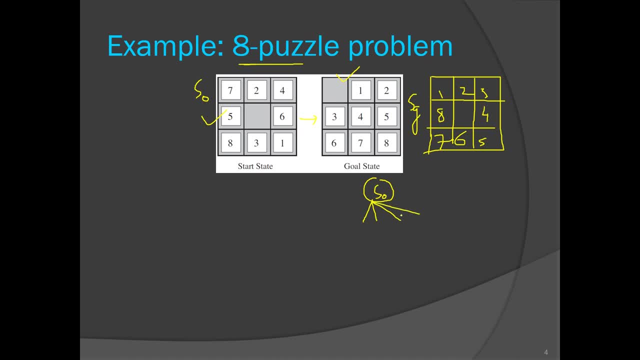 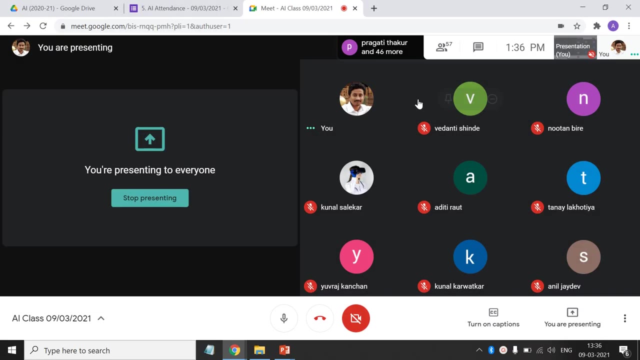 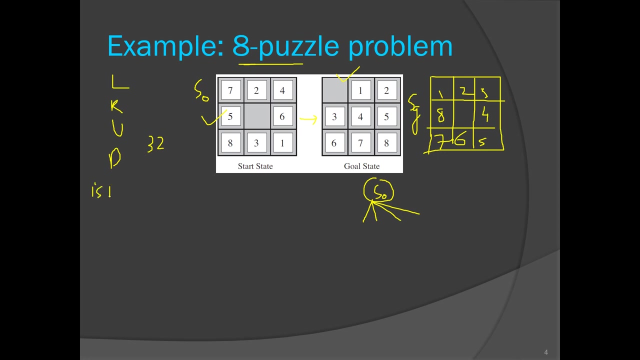 actions are possible for me from this S0?. So now for each tile I can move that tile to left, right up and down. So 4 actions are possible for this 8 tiles. That means I have total 32 actions. So for first tile I have left right up and down. For second, 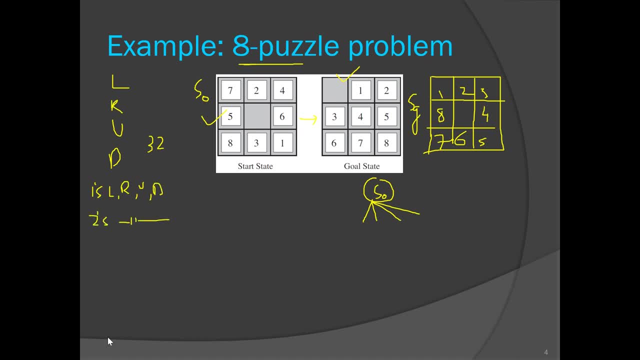 tile, I have again same thing. So in total I have 32 actions. So now, can I move this? can i reduce this number of actions from 32 actions? can i reduce this actions? so now, when i am moving, when i move tile number 5- ok, you look at this blank space. ok, blank space- can. 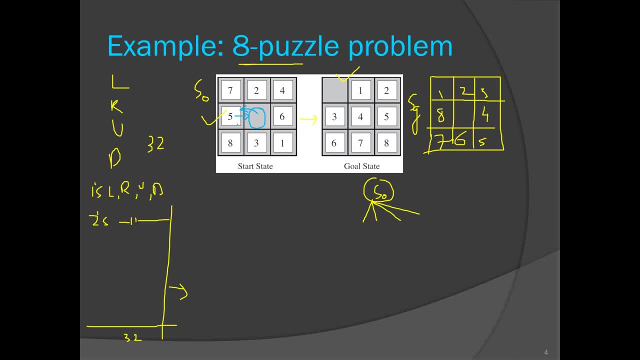 i say that blank space is moving towards left. ok, when i move any tile, ok, so blank space will be moving right. so if i mention the action in terms of blank space, so i can say that blank space is moving towards left, to moving towards right and up and down right and in. 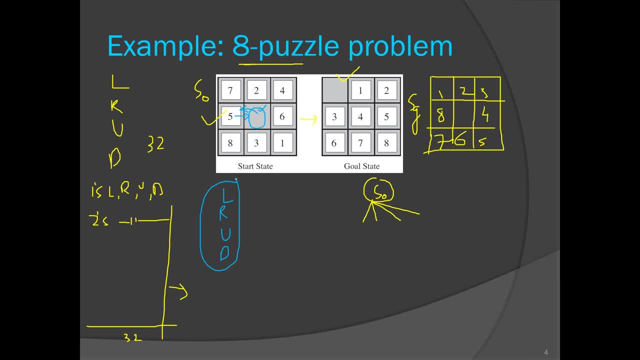 any move. ok, blank space will ultimately move. ok, if i move this 6 to the left, blank space will move towards right, right. so instead of specifying the action in terms of this number, number tiles, i can specify the action in terms of this movement of this blank space. ok, so 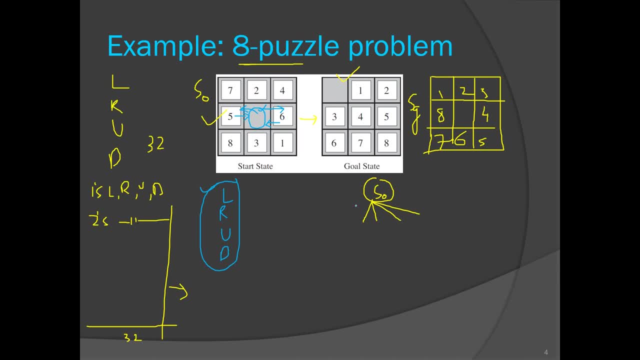 now, from s0, my blank space can move towards left, right, up and down. ok, so now, if i move a blank space towards left, which configuration i am getting? so my blank space is moving towards left. that means 5 will come here and rest of the tiles will remain as it is. ok, so this is the state. 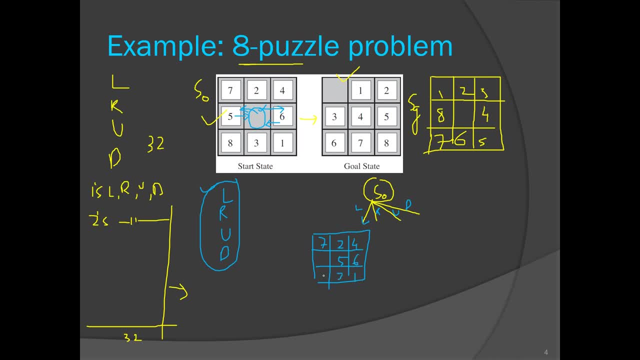 i am getting right. ok, now let let me call this state as s1. ok, now, from this s1, how many actions are possible? now, blank space cannot move towards left. ok, so only three actions are possible. so, right up and down. if i move right this blank space to the right, i will be waiting again. s0- ok, same state. i. 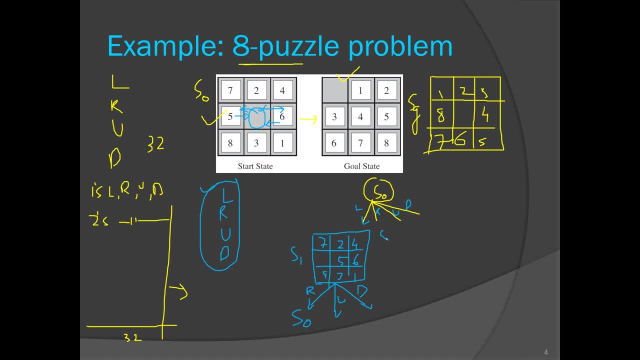 am getting ok. so and if i take a right move here at the s0, i will be getting s2, s3 and s4. ok, so in this way, when i am searching for a solution to this problem, ok, i am getting a tree like structure right and this: 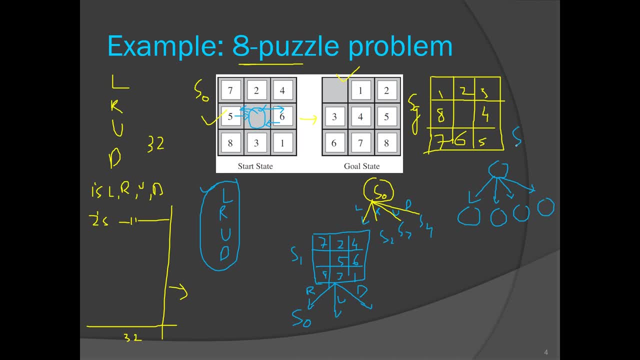 tree is actually known as search tree. this is known as search tree and our agent will be searching for a solution in this search tree, ok. that's why our the title of this unit is solving the problems by searching ok and how our agent travels through this search tree. ok defines the different search. 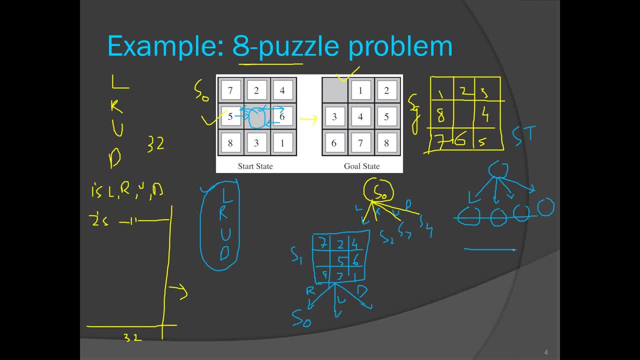 strategies: ok. whether he is going going by level, by level, then it will be bfs. whether he is going by charge, that will be a dfs, and so on. ok, so when such tree is formed, that search, that tree is known as search tree. ok, the collection of states in this search tree is known as state space ok collection. 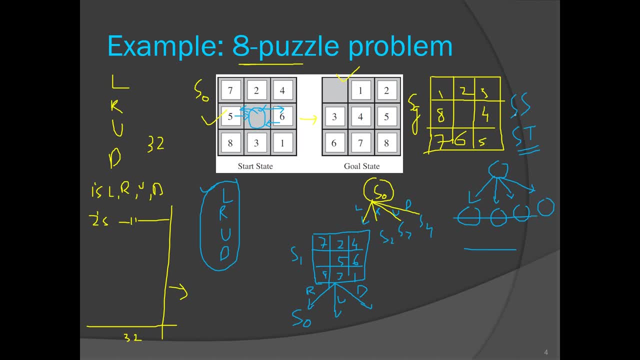 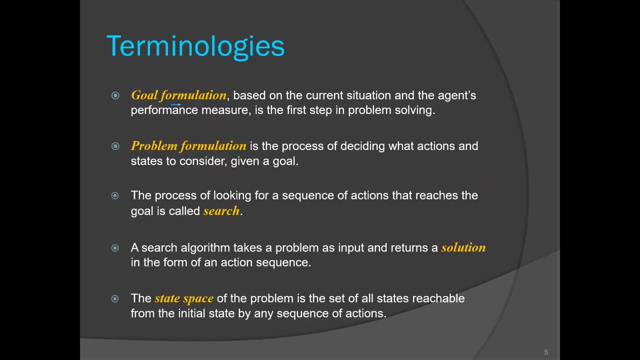 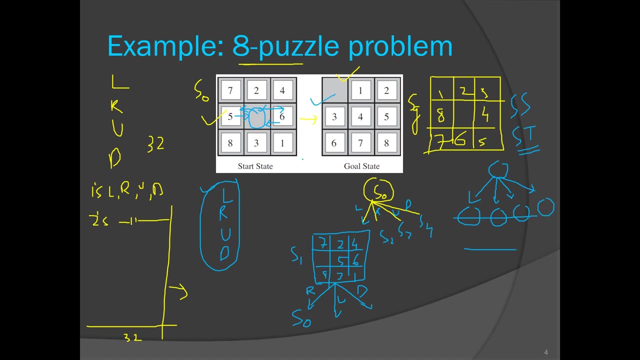 of all the states formed in the search tree are known as state space. ok, so now let us try to understand different terminologies. so first one is goal formulation. when you formulate any goal in terms of a performance measure, ok, so what performance measure we want here? our agent should. 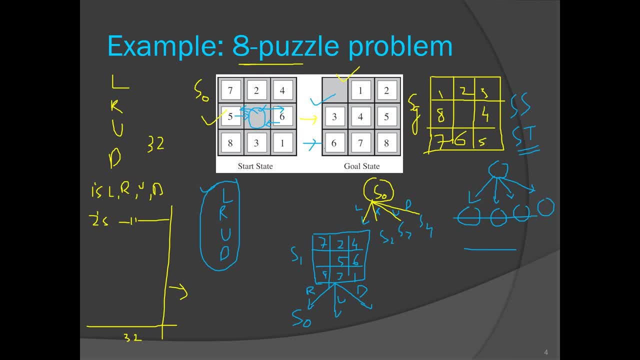 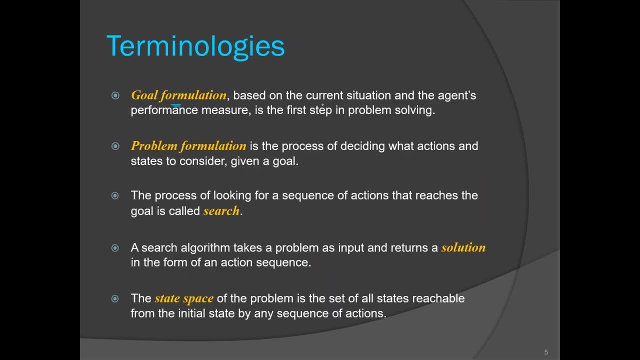 move to this goal state in minimum number of moves. right, that is my performance measure. i should get this goal state. ok, but in minimum number of moves. so this goal formulation is the first step in problem solving. first you have to formulate the goal, because our agents are goal based agents. 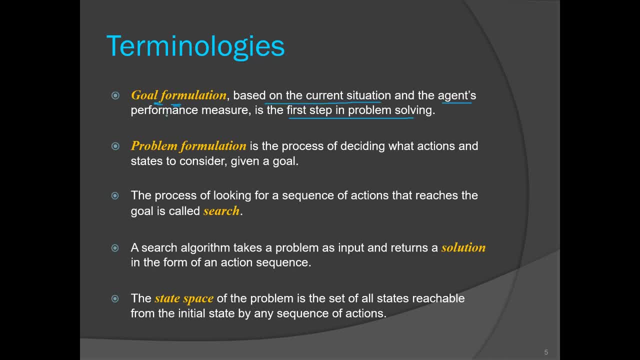 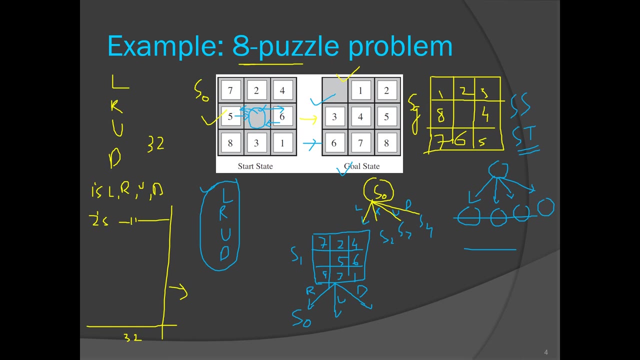 right. so, based on the current situation and the agents, performance measure. Goal formulation is the first step in the problem solving. So first terminology to remember is goal formulation. Next one is problem formulation. So in order to formulate this problem, we will find out how many actions are possible. So here we. 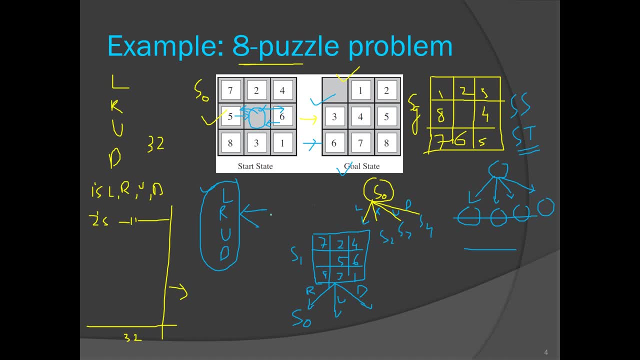 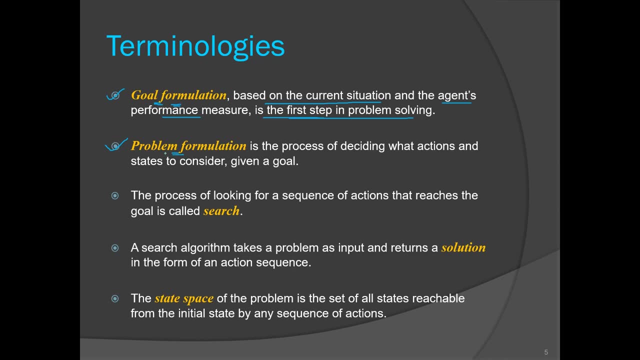 have found out all the actions possible, Then how many states are possible. Based on that, we will formulate the problem. So what do you mean by problem formulation? Problem formulation is the process of deciding what actions and states to consider given a goal, So we may 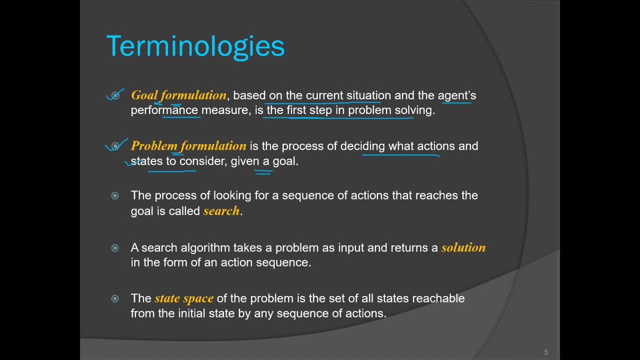 exclude some states. We will see some problem where we will exclude some states which are not favorable. Next one is search. So we have obtained a search tree, So our agent will be looking for a solution. So we have obtained a search tree, So our agent will. 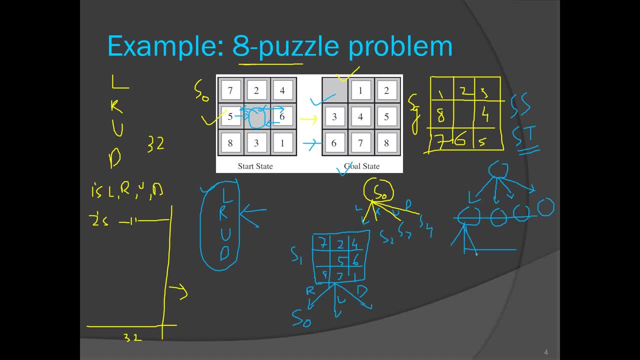 be looking for a solution. So if you follow this tree Now, if you see here, our root node of this tree is our initial state or a start state, and at the leaf level, at the end, we will have our goal state. We will reach to the goal by following different paths. We 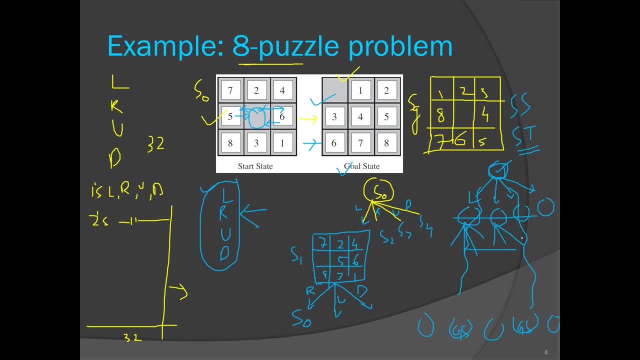 may reach to the goal state by following different paths. So we may reach to the goal state by following different paths. right, so these are different solutions to our problem. okay, and what do you mean by solution? so, from the root node, if i apply this sequence of action, i will reach to. 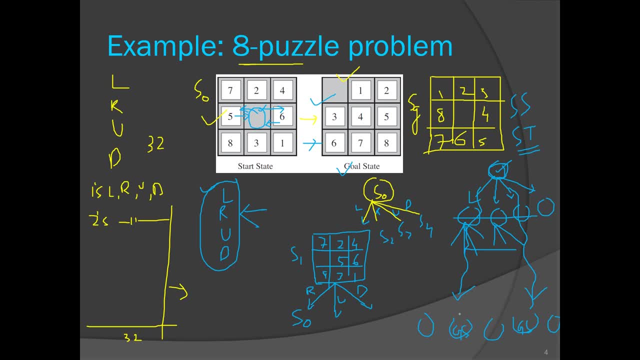 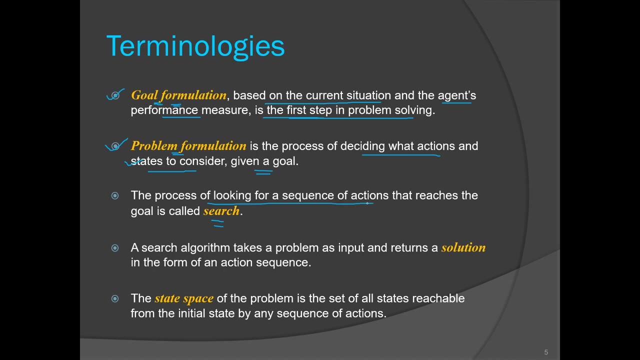 the goal state and that will be my solution. okay, so solution means what a sequence of action to reach to a goal state is a solution and process of looking for that is known as search. okay, so see the definition of search: a process of looking for a sequence of actions that reaches to the 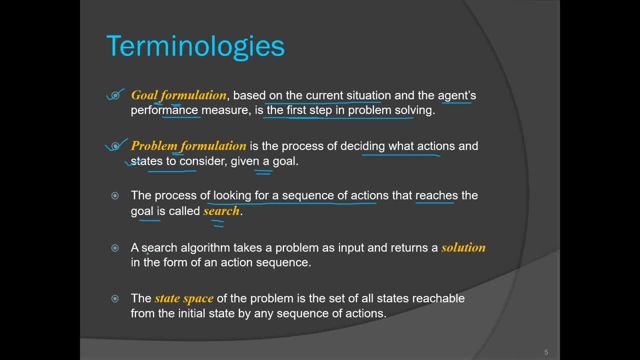 goal is called a search. okay, and a search algorithm takes a problem as input and returns a solution in the form of action sequence. okay, so solution will be a set of actions. okay, sequence of actions. now we talked about state space also, right? state space means what? the collection of 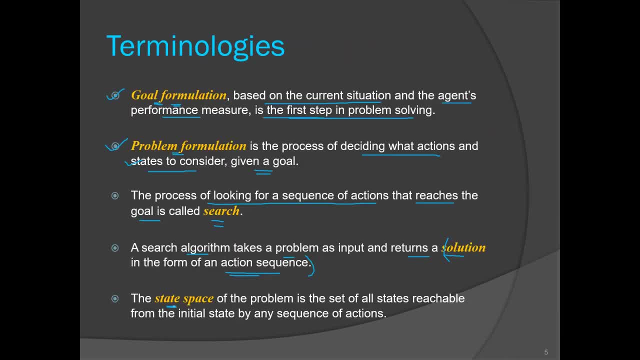 this sequence of actions will be a set of actions. okay, so the collection of this sequence of actions is known as state space. okay, so state space of the problem is a set of all state reachable from the initial state by any sequence of action. okay, so you apply all the possible actions on any state. 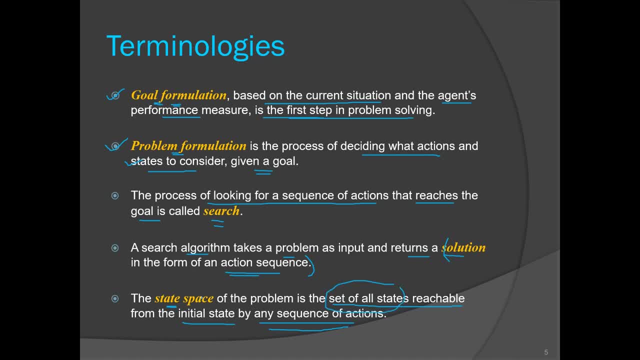 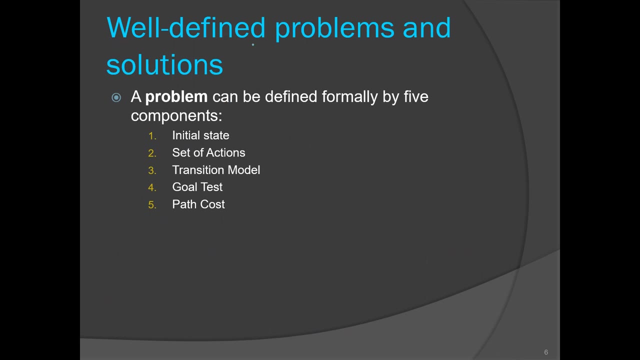 okay, and you will get a set of states. okay, and that is known as state space. so i think the terminology is clear to you, okay, so try to remember this terms now. um, so, now our agent will be solving our problems right, so your problem should be unambiguous there. 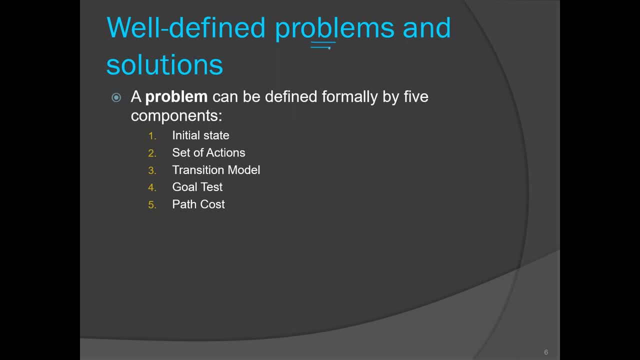 should be no ambiguity. that means there should be no confusion to our agent. okay, so it is said that your problem should be well defined. okay, so there should be no ambiguity in the problem. now how to avoid that? so if you specify your problem in terms of these five components, then we we can ensure that. 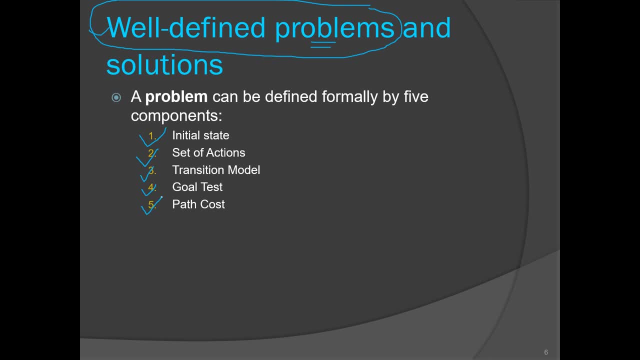 our problem will remain the same. okay, so now let's talk about the problem. so let's talk about the problem: unambiguous. okay, so we will state our problem in terms of these five components. okay, so they will try to cover all the aspect of your problem. okay, so here we are not concerned with the 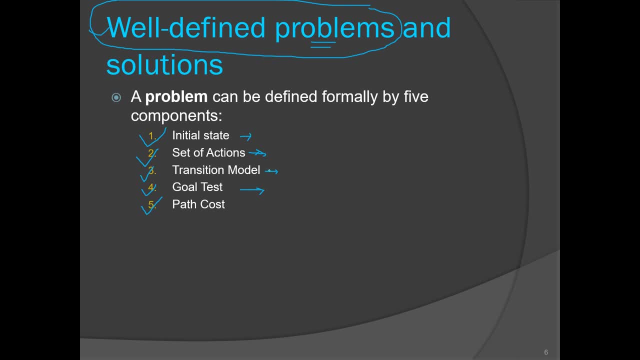 solution. here we are trying to define our problem in unambiguous way. okay, so what are those five components? so we have initial state. okay, so what is the initial configuration? what is the starting point of my problem? okay, just like this. so this was my initial state. okay, so what is the initial? 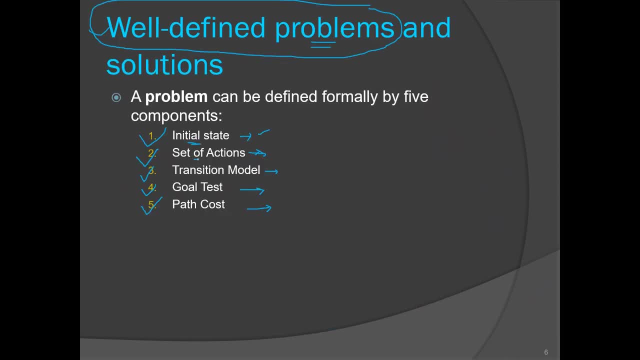 state, right. then next one is set of action: okay, so possible actions available to our agent. then transition model: okay, so this transition model is actually a function. okay, a function on state and action, okay. so. so what is the meaning of this function if i apply this action on this state? 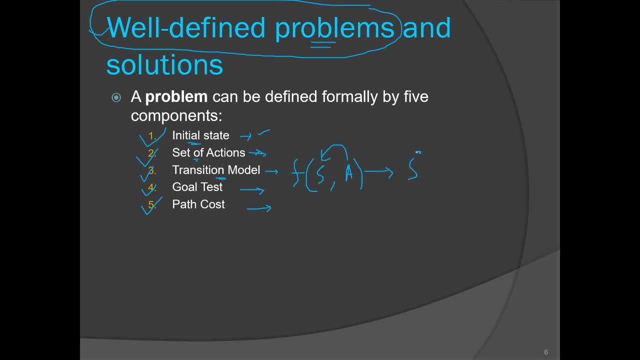 which state i am getting. okay, so i will be getting a new state, okay. so that is governed by this. this transition is governed by this transition model, for example, in our previous uh example. so s0 was my initial state and if i apply a left action on that, i was getting s1 state right. such transition. 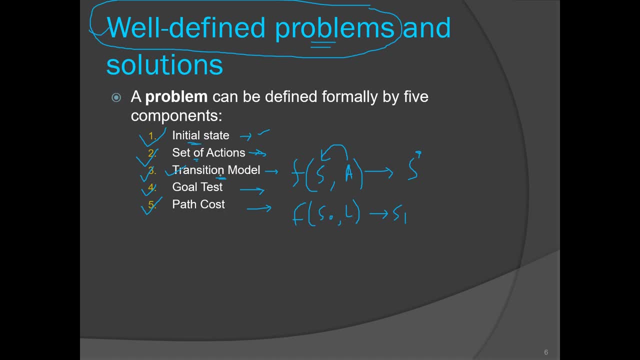 will be governed by this transition model. okay, so this is a function. remember that. now gold test. now, this gold test is actually a boolean function called g and this we will apply a state. okay, now it will return true and false. okay, if my current state okay, denoted by s if it. 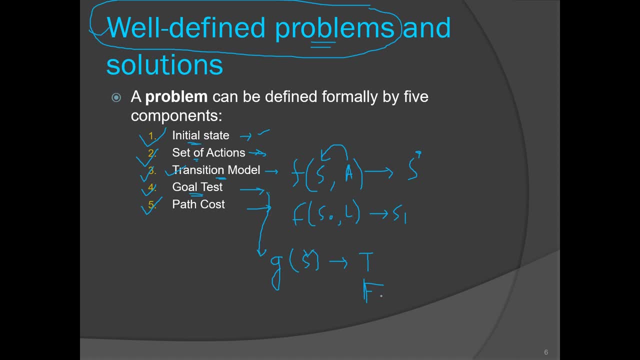 is a gold state, it will return true. otherwise it will return false. okay, so whether my current state is gold state or not, that can be determined using gold test. okay, next one is path cost. okay, so here this path cost means the cost assigned to the solution. okay, so in previous example, 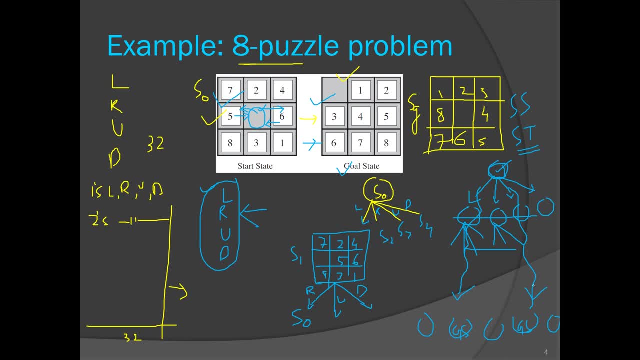 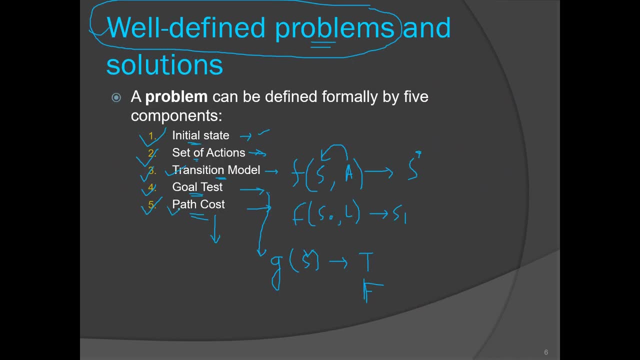 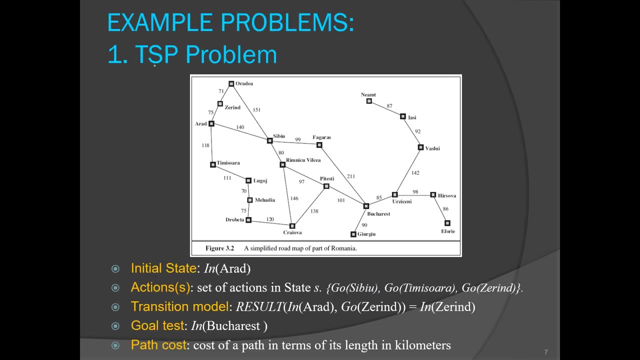 path cost can be number of moves taken by the agent to the to reach to the gold state. that will be the path cost. okay, so we want that solution with the minimum path cost. right? so this? these are five components, so we'll see some example problems. i will start with traveling sales salesman. 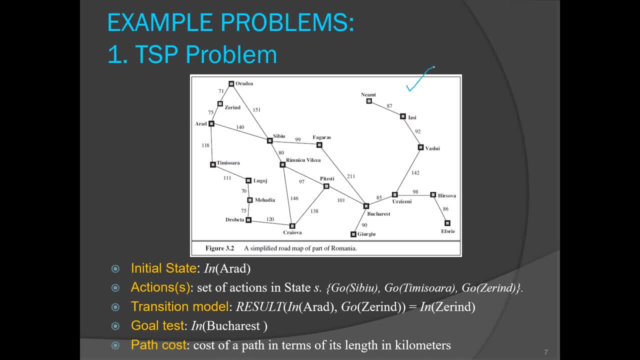 problem. okay. so now this map is of romania country, okay. now our agent is located in arad uh city, okay, and his destination is this: bucharest. okay. so now he wants to go from this arad state- sorry, arad, maybe it is city- so from arad city to bucharest city, okay, so we can see that this is one. 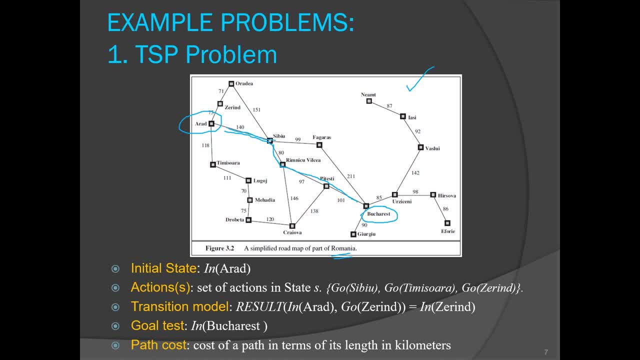 uh solution: okay, another solution is this one: okay, so this will be two different uh branches in our search tree. right, this is another one possible path. okay, and we want the efficient- sorry, the- the path with minimum number of kilometers. okay, so these numbers are actually a kilometer, okay, distance in terms of kilometers: okay, so now. 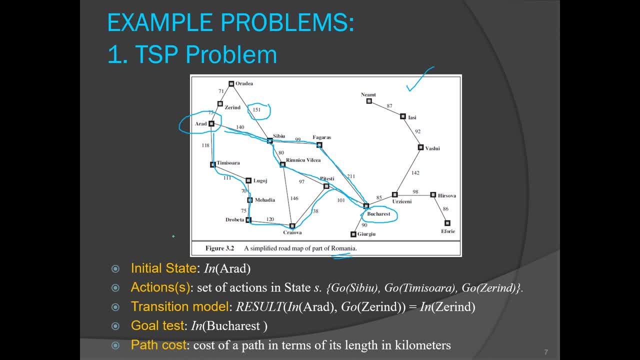 we'll try to define this problem okay in terms of those five components. first one is initial state: okay, so initially my agent is in arad, right, so i am indicating that with the function called in. so my agent currently is in arad, okay. next actions: okay, so now, at this moment, 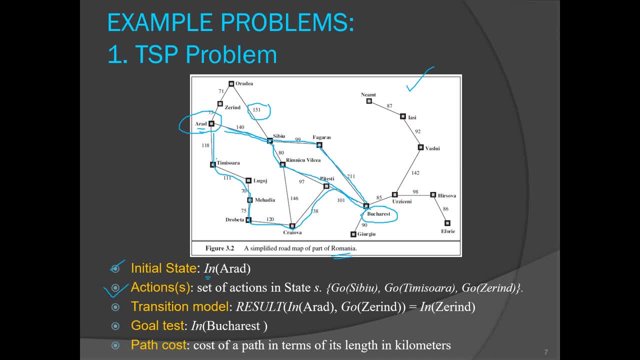 how many actions are possible to me? okay, so, at this, uh, at this state, our agent may go to cbu. so this is one: uh, city, cbu, then team is sora and then zherind, zherind. okay, so these three actions are possible at this state. okay, so this will be my set of actions. okay, so i am indicating. 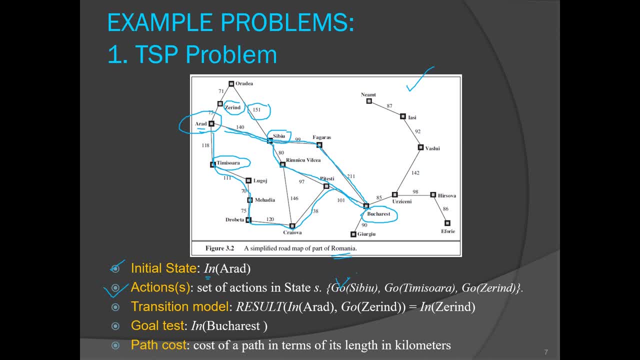 that action, with the help of this, go function. so from this arad state he may go to cbu or team is sora and or zherind. okay, so these are my set of actions. then transition model: okay, so now this is our function, right? so if my current state is arad and my action is go zherind, okay, this is my action. 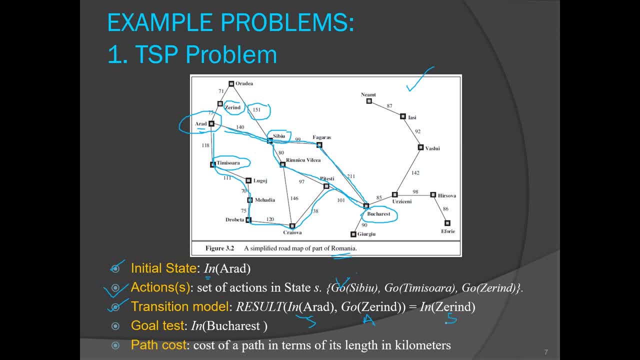 okay, i will reach to zherind right, so this will be my new state, indicated by in zherind. okay, so from arad, okay. so my current state is in arad. my action is go zherind, so result will be in zherind, okay. 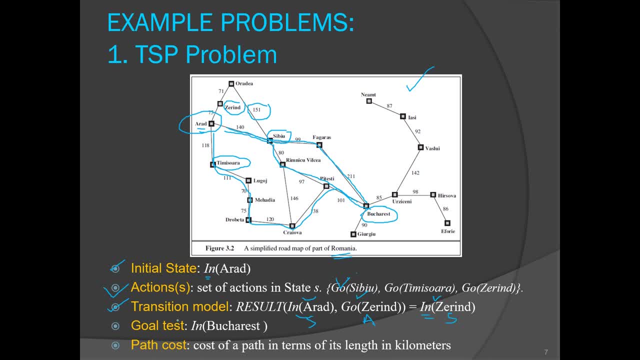 that will be a transition model, okay, so we have to define this, uh, transition for every possible combination. okay then goal test. okay, so my agent should reach to book arrest, right, so my goal test should will be in book arrest, right, both goal state- sorry, goal state- will be in book arrest. now, path cost: cost of a path in terms of its length in kilometer. 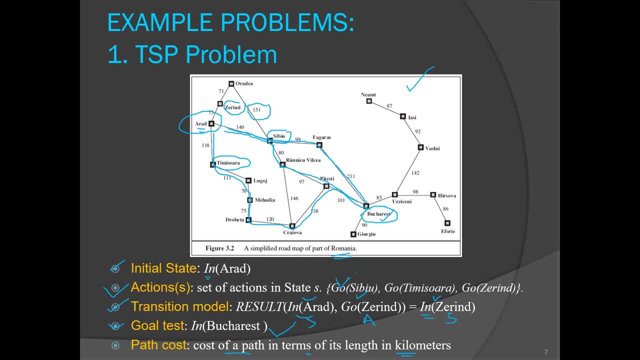 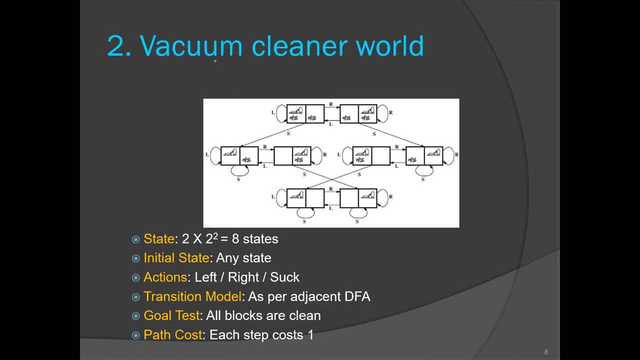 okay, that will be my path cost. okay, so path cost for this path will be different for this path will be different. okay, so this is: this is how i can define this tsp problem using this five components. uh, let us see our vacuum cleaner world. okay, so how to define this problem now, how many states are? 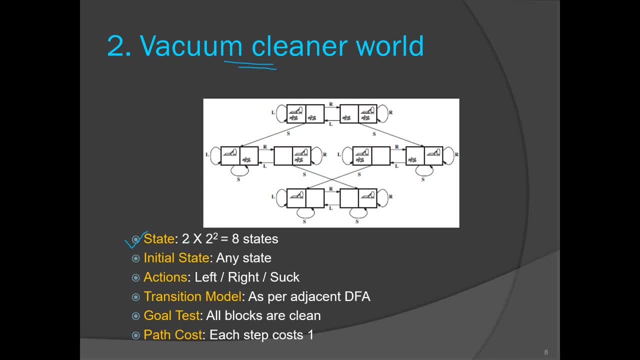 possible. so we'll find uh, we'll find different states possible. so now uh this: so we know that we have two blocks and dust may be present at both the blocks- okay, or it may be present in only uh block b- okay, or block a, and we may have uh clean. 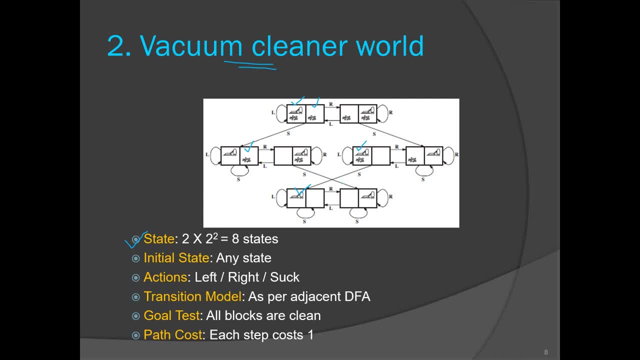 uh, clean blocks. okay, so this is four state possible and our vacuum cleaner can be present in block a and block b. okay, so multiply by two that means eight states are possible. okay, so four combination for dust and two combination for the placement of the vacuum cleaner. so total eight states are. 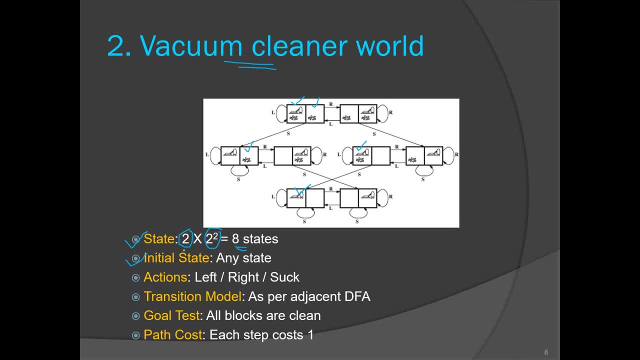 possible now. initial state: okay, so your agent, your system, may start with any state. okay, out of this, any one can be the initial state. now, what actions are possible to our with our agent? so left, right and suck, okay. so now see here if we start with this configuration. okay, let me call this as s0. 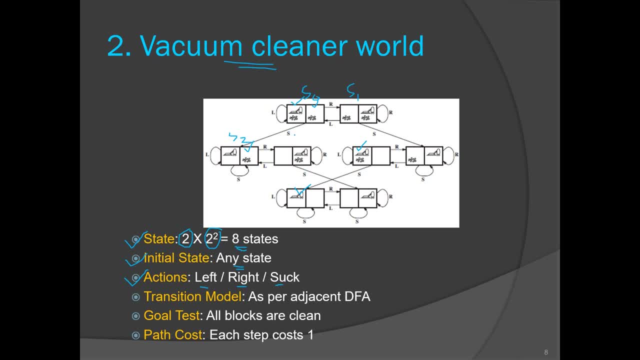 this is s1, s2, s3, s4, s5, s6 and s7. okay, so these are my states. i am starting with s0. if i issue a command left, okay, so now he will remain in that that state only right now. if i issue a command r, i will move to s1 state. now, here, if i execute a command, suck. 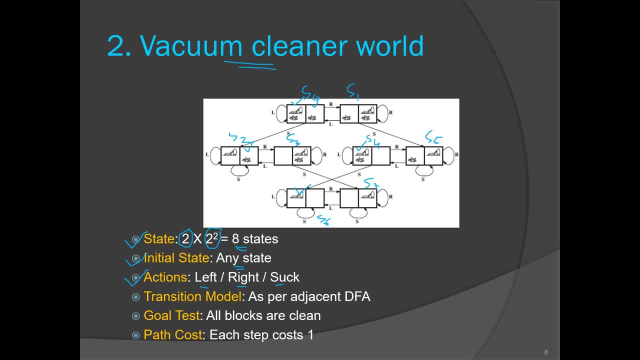 okay, i will move to state 5: right, and that floor will be clean right now. here, if i execute a suck command, i will remain in s5 only, right, because the clear, the floor is already clean, right. so now, on every state, i am writing- uh, writing this- possible actions, right, and i am determining. 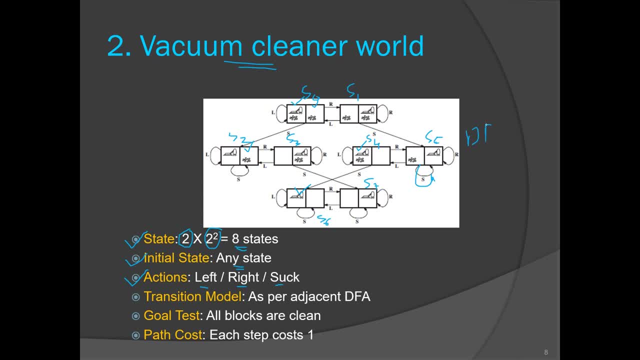 new states. okay, and this is actually a dfa right- deterministic finite automotive right. okay, so now, what will be my transition model? okay, so now, if i'm in s0 and if i execute a suck command, which state i'm getting? now this can be determined by me after i execute the而 i 648, which state i am getting. 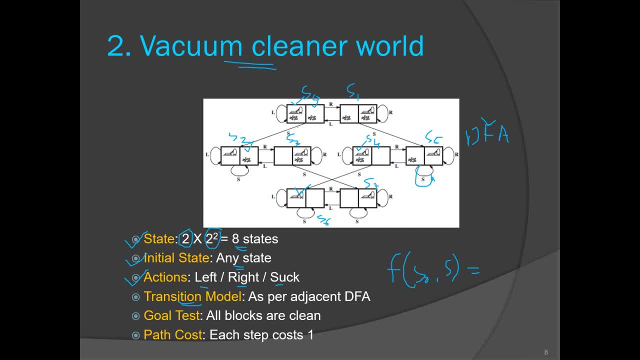 with the help of this dfa. right, i am in s0 and i am executing suck command. i am going to s2. okay, so it will be as per the adjacent dfa. okay, so from this transition diagram, i can determine my transition model. okay, then, what is my goal test? okay, ultimately, why? what we wanted in our 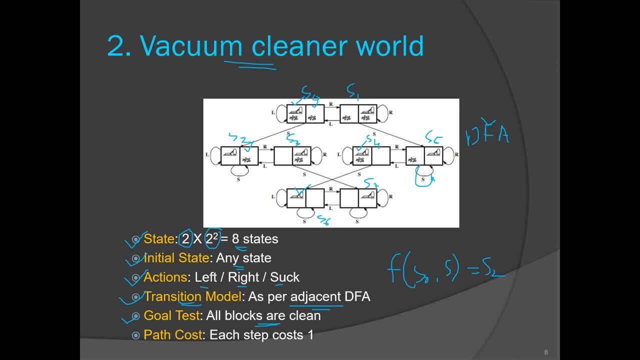 system. all blocks should be clean. right, that will be my goal. test now path cost: each step will cost me one unit of something, right, one unit. so if i start with s1, state what will be my path cost. okay, so now the most efficient path will be this one. okay, i will issue. 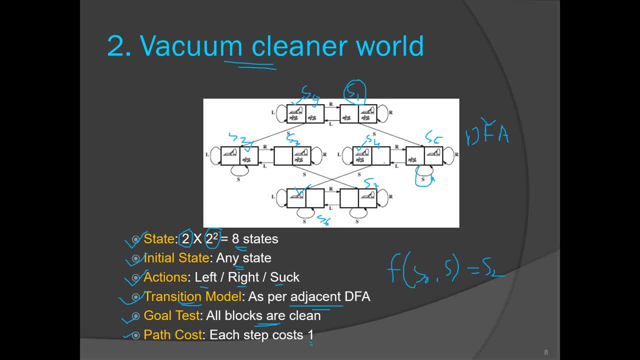 a suck command here, okay, and then left command, okay, and then suck command, okay. so in three actions i can get a. i can reach to the goal state, right, so suck command will clean this floor. then left command will bring me to the block a, and then again suck command- right, so that will. 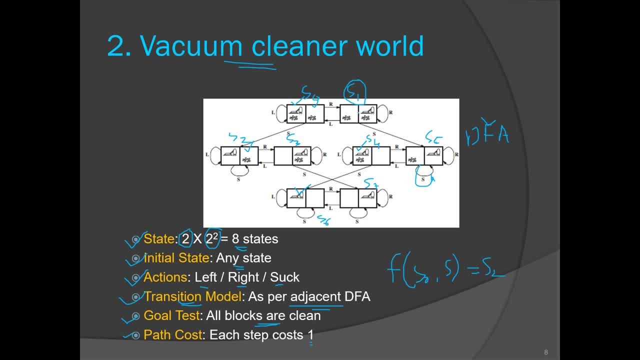 be my path cost. our agent may reach to the goal state by following different path, also here itself. he may issue a left command. okay, so, let me change the color of pen. okay, so if, okay, i am starting with s1. okay, he, if he goes to left, okay then suck command. okay, then right. 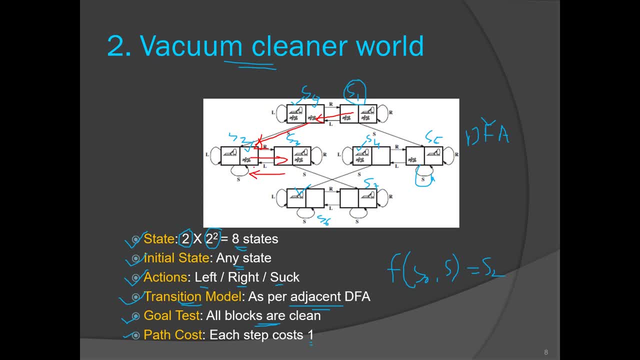 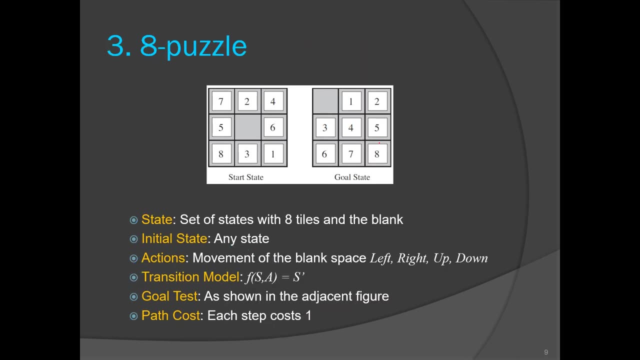 unnecessary. he may issue a left command and then again right command and then suck command. so in this case, what will be the path cost? one, two, three, four, five, six, six. okay, so we may reach to the goal state by following different paths also okay. now next example is eight puzzle problem. 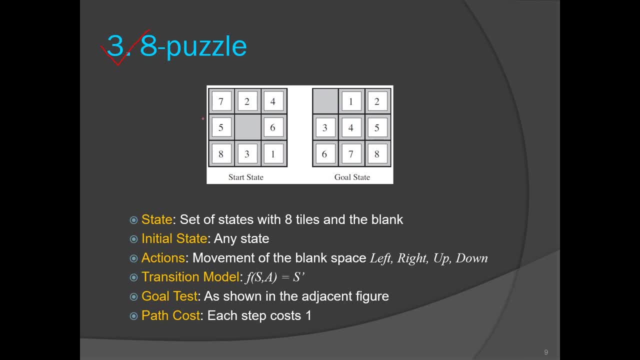 okay, so we have discussed this. okay, so let let us try to define this problem. so state, okay, so what? what is, uh, what are the different possible states here? set of states with eight tiles and the blank? okay, so any possible combination of this- eight tiles and the blank- will be our set of states. 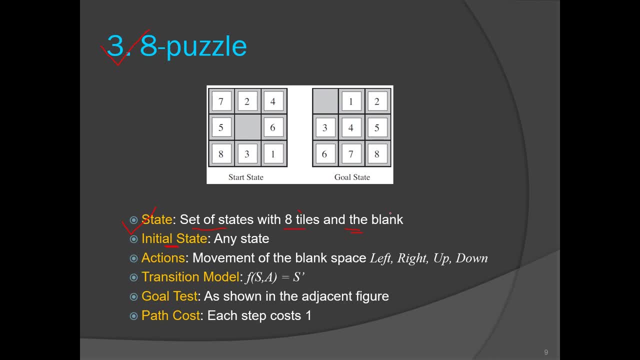 right then, initial state: any state out of this. so let me show: represent this set of states by capital s. any state small s belonging to this capital s will be my initial state right now. actions: so we are mentioning, uh, the action in terms of the movement of blank space. right, so, movement of blank space. 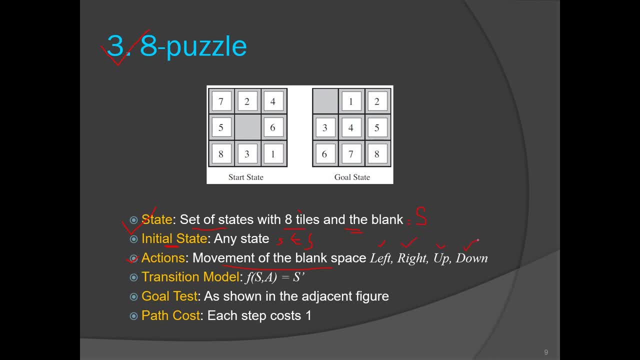 it can be left right, up and down. then transition model: okay. so again. so if i apply this action a on s, i will get a new state. okay, so that will be my transition model goal test. so goal test will be as shown in the adjacent figure. this is my 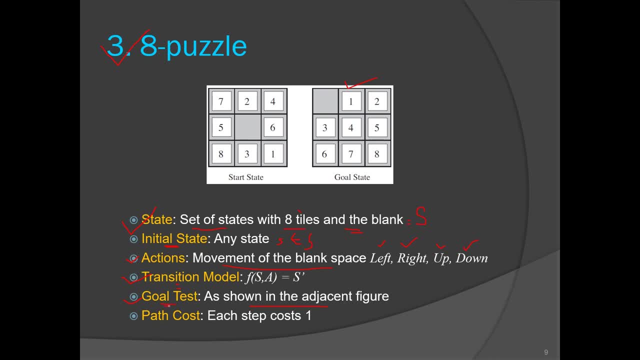 goal state: okay, so goal test will compare whether my current state s is equal equivalent to this, my this sg. okay. whether my s current state is equal to sg. okay, so goal test will compare that. and path cost: each step will cost me one unit, okay. each movement of tile will cost me one unit. that will be my path cost. 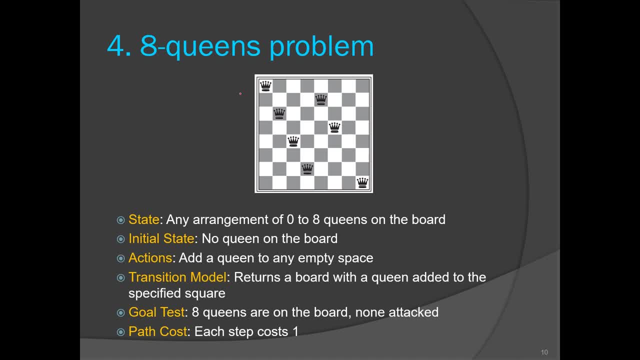 now next problem is eight queen problem. okay, so what is the problem statement here? so here we want to place eight queens on the chessboard. so we know the dimension of chessboard. it is eight by eight, right, eight by eight, eight by eight, okay. so now we want to place eight queens so that no two queens. 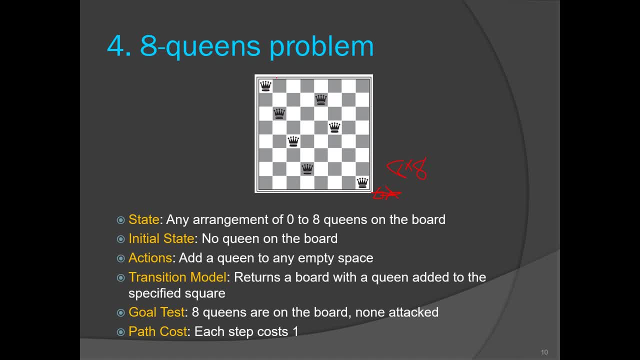 each other. now, this is not the final solution, because this, this queen is actually attacking this queen. okay, so this is a partial solution. so this is the eight queen problem now. so what is the state here now? so initial state is actually: no queen on the board. okay, so we'll start with the empty board. 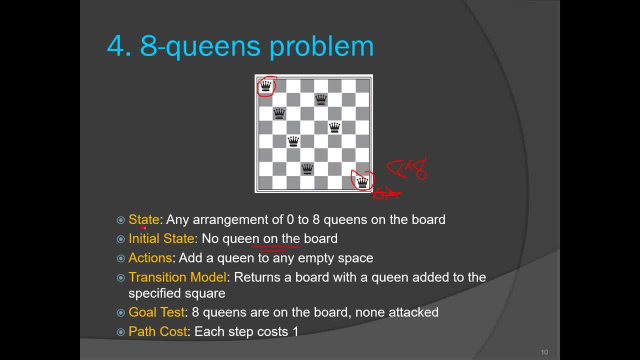 okay. so what are the possible states here? any arrangement of zero to eight queens on the board, okay, be uh case where uh queen are attacking each other, okay, but that will be one one of the state, right. so any arrangement of zero to eight queens on the board will be my state's space, right then? initial, 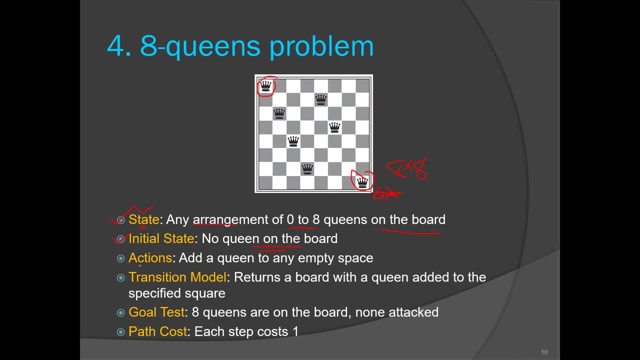 state no queen on the board is my initial state actions. okay, so every time i will add one queen to the empty space. okay, every time i will add one queen to the empty space, then what is my transition model? okay, so when i place a queen, it will return a board with a queen added to the specified square. 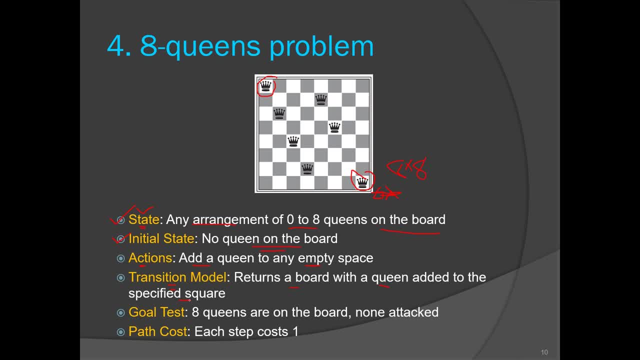 okay, that that's how our board is going to change. right, that will be the transition. then gold test: what is my goal test? ultimately, i want eight queens on the board, none attacked. okay, no one is attacking anyone. right then, path cost: each step, each placement of the queen will cost me one. 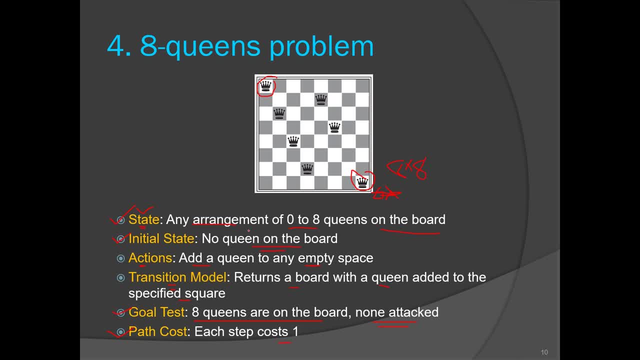 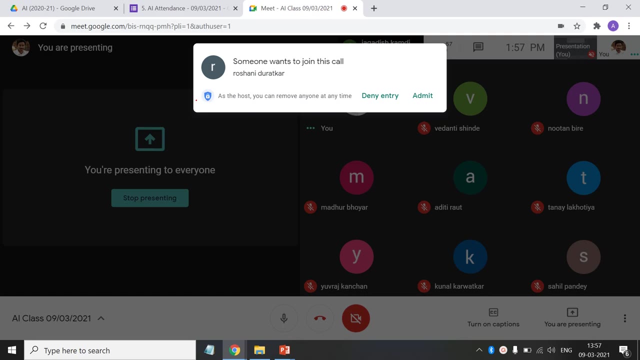 okay, so this is eight win problem. okay, so now, currently we are not concerned with the solution, we are just trying to define our problem. okay, we are trying to define all aspect of our problem now. last problem is three missionaries and three cannibals. okay, so this is our homework problem. 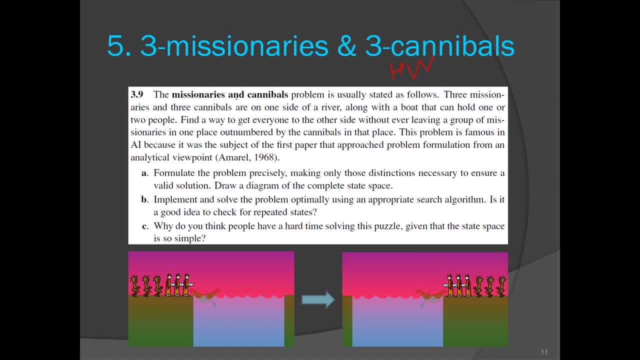 now, what is this problem? so here we have three missionaries and three cannibals- okay, and they are on one side of a river- this is our river- and they have one boat- okay, but the capacity of this boat is it can carry either one or two, not more than two, okay- and they want to cross this river. 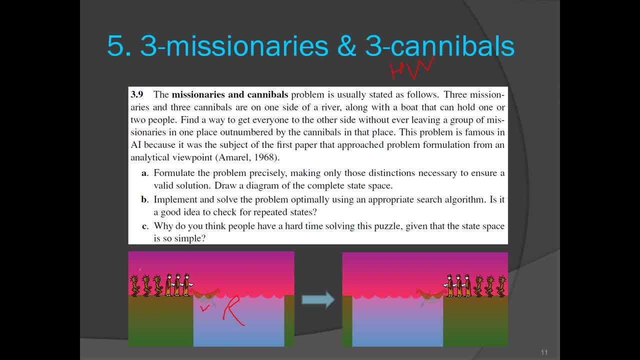 but the condition is that if this cannibal, the number of cannibal, becomes more than missionary, those cannibal can kill the missionary. okay, so if, at one particular moment, if you have two cannibals and one missionary on one side of a bank on the river, okay, these two cannibal can kill this one. 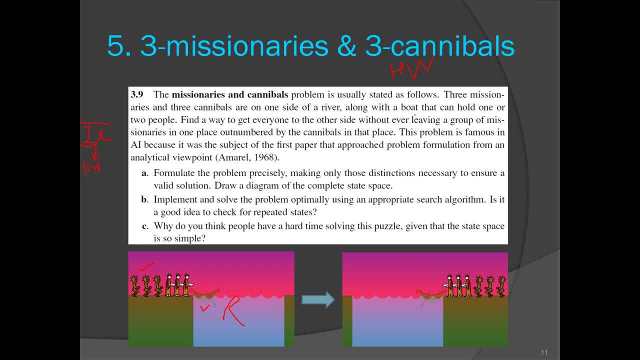 missionary. okay, so read the problem statement here. three missionaries- and three cannibals are one- are on one side of a river, along with the boat that can hold one or two people. find a way to get everyone to the other side without ever leaving a group of missionaries in one place, outnumbered by